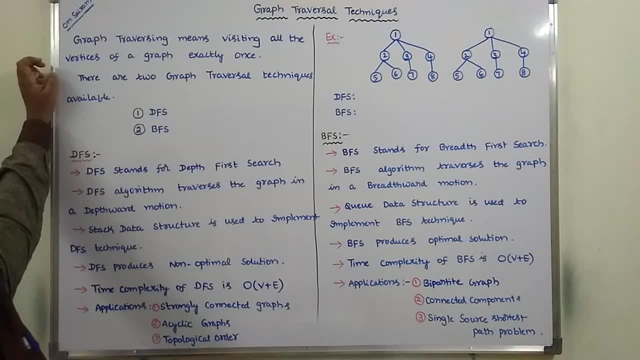 There are two types of graph traversal techniques are there. First one is BFS and second one is DFS. Okay, in the same way, tree traversal techniques are also there. Tree traversal means visiting all the vertices of a tree exactly once. It is nothing but tree traversal. There are three types of tree. 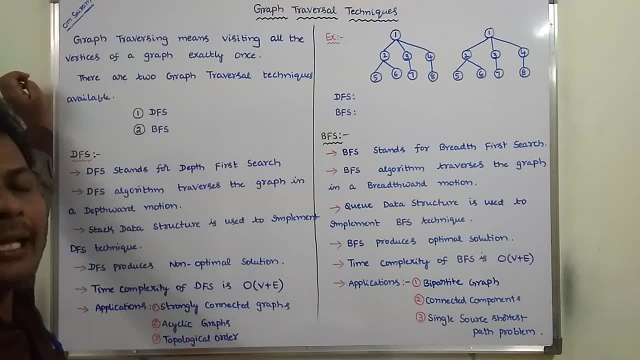 traversal techniques. First one is BFS and second one is DFS. There are two types of graph traversal are there? first one is pre-order, second one is in order and third one is post order. okay, next one. so, among the two gravel techniques, graph traversal techniques. first one is dfs. first point: 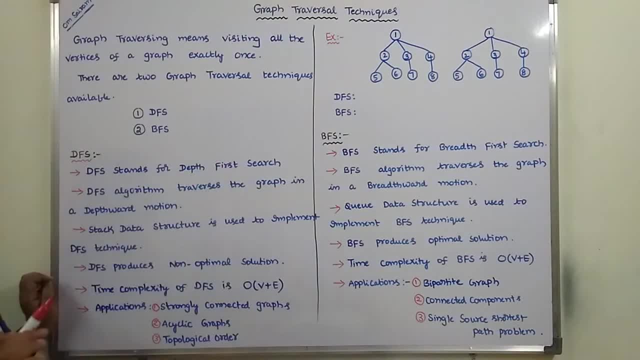 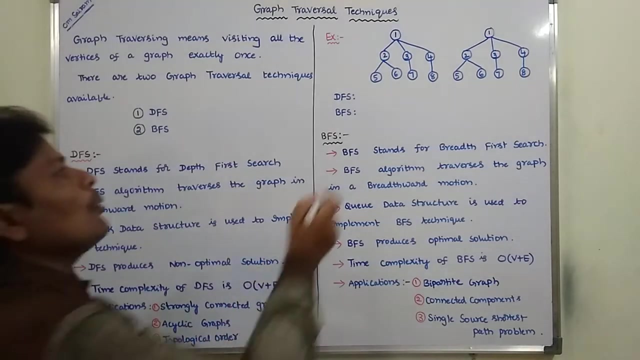 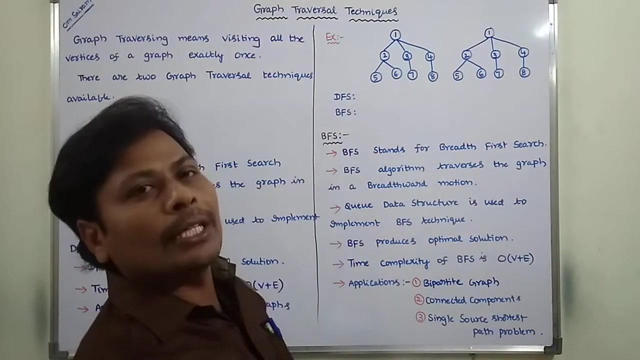 bfs stands for depth, first search, next one bfs algorithm, which is all the vertices of a given graph in a depth world motion. so what is depth word motion? now consider this graph. this graph contains eight vertices. okay, these eight vertices are visited in a depthward motion by 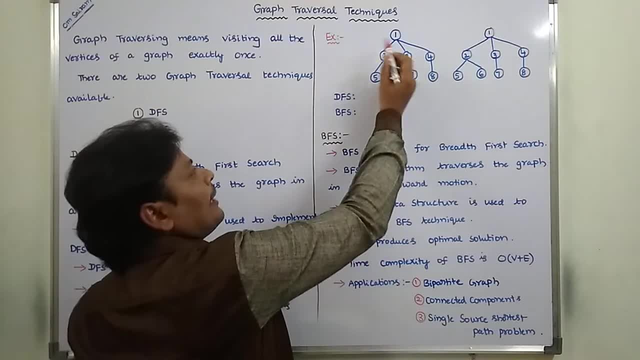 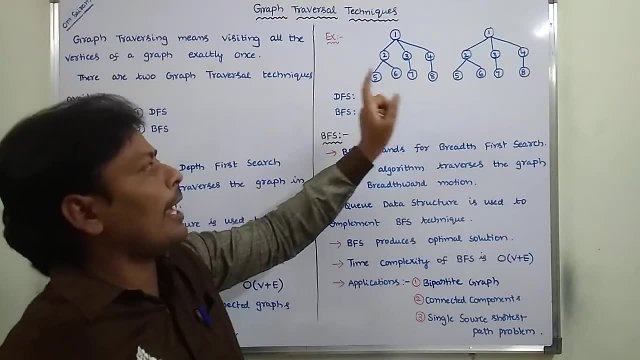 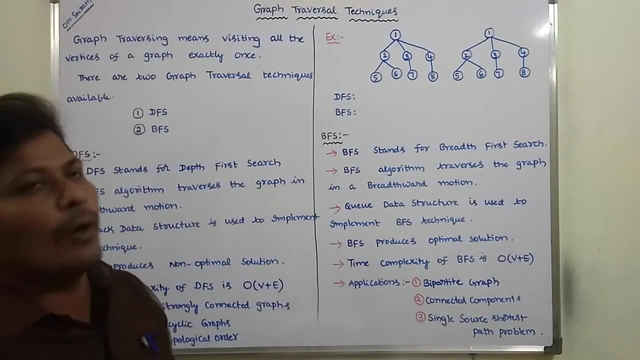 using dfs, DFS. Okay, In the DFS, we are starting at any vertex. We are starting at vertex 1 or vertex 5, or vertex 7 or vertex 8.. We can take any vertex as a starting vertex. Okay, I am taking vertex 1. 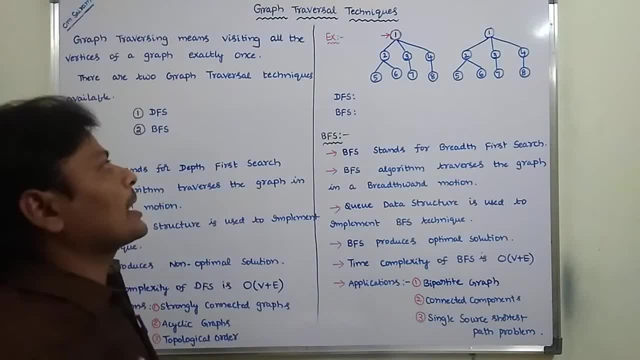 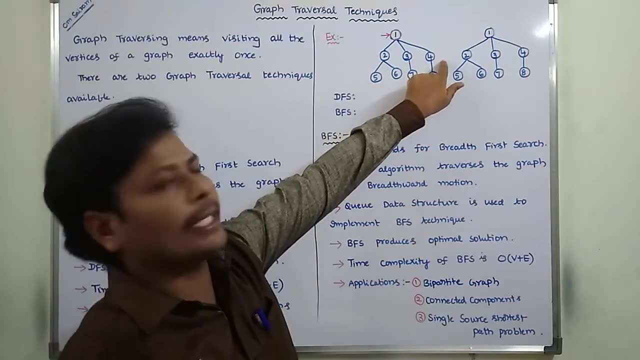 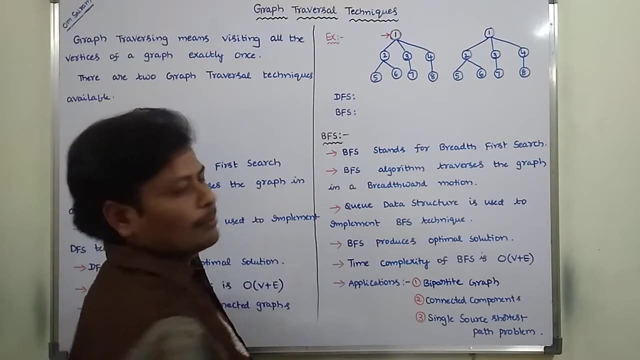 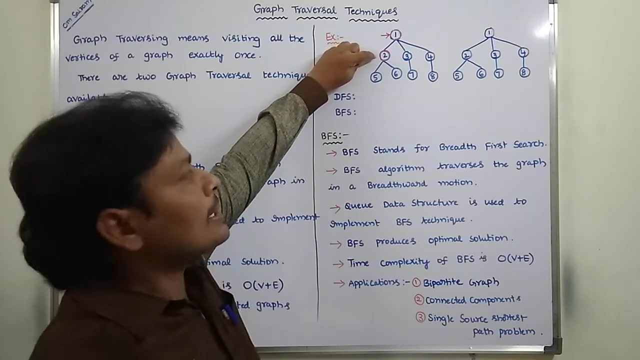 as starting vertex. Okay. Next one For vertex 1,. what are the adjacent vertices of the vertex 2, vertex 3, vertex 4?? These are the adjacent vertices of vertex 1.. Among them, we are taking any vertex. Okay, So I am taking vertex 2.. Okay, Now consider vertex 2.. What are the adjacent? 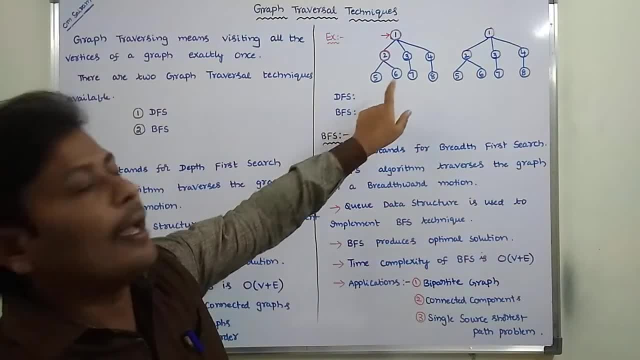 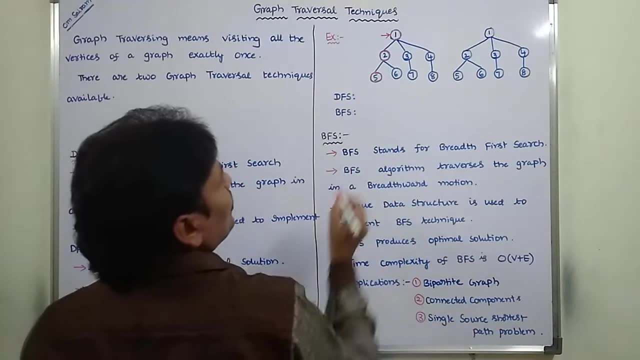 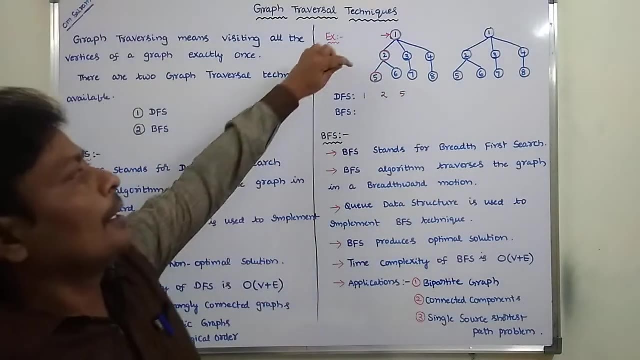 vertices of them, That is 5 and 6.. Among 5 and 6, we are taking one vertex, That is 5.. So first I am taking vertex 2., Taking 1, then go to 2, then go to 5.. Next one, Now consider the vertex 5.. What are the adjacent? 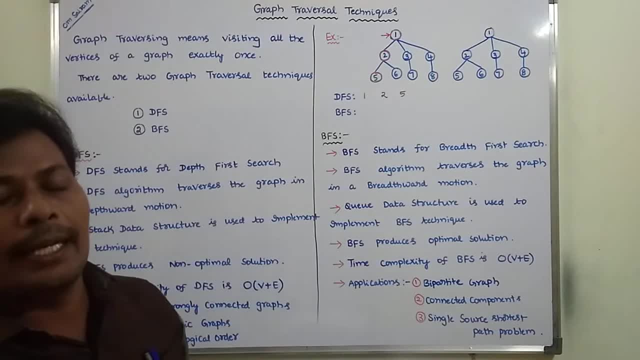 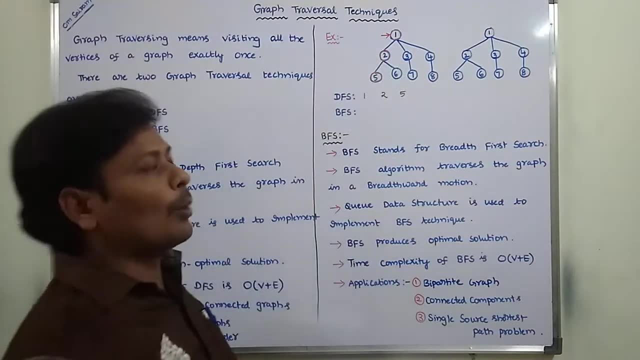 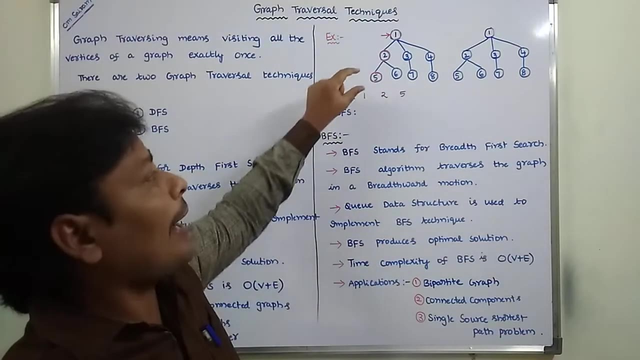 vertices of it. There are no vertices of it. That is adjacent to vertex 5.. Again, we have to backtrack to vertex 2.. Now vertex 2, what are the adjacent vertices? 5 and 6, but 5 is already visited Then. 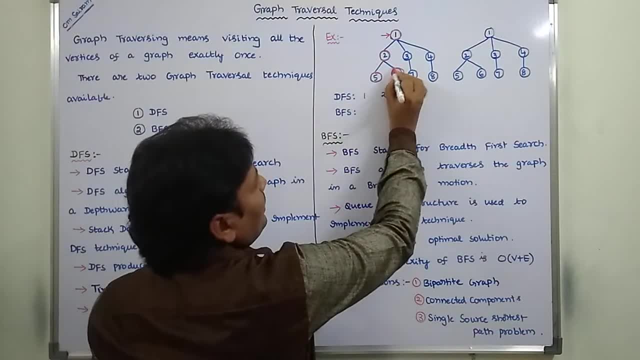 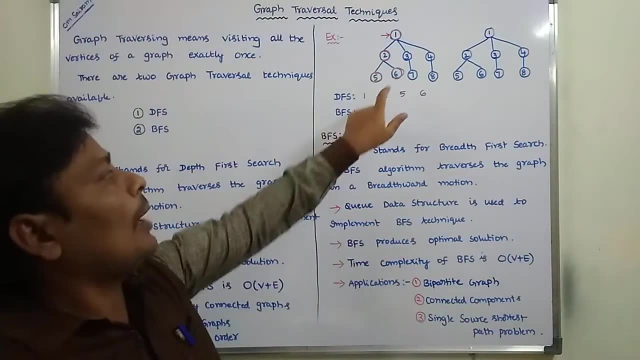 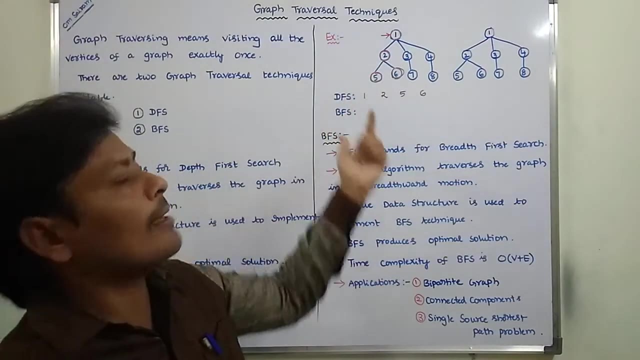 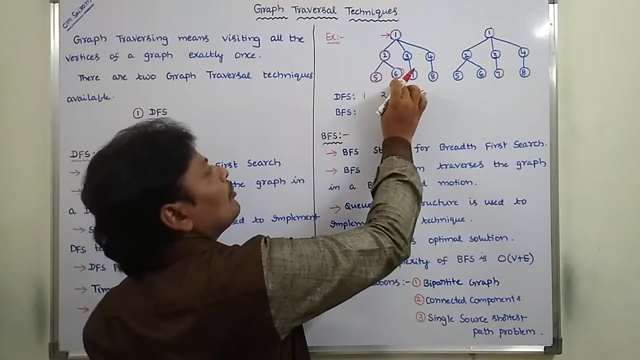 visit vertex 2.. Now vertex 2, what are the adjacent vertices? 5 and 6, but 5 is already visited. Then visit vertex 2.. Next one, Now vertex 6.. Now vertex 6 is visited. Next one: Now consider vertex 6.. What are the adjacent vertices of vertex 6? Only vertex 2 is there, but 2 is already visited. So there are no adjacent vertices for vertex 6.. So again we have to backtrack to vertex 2.. Okay, Next one. 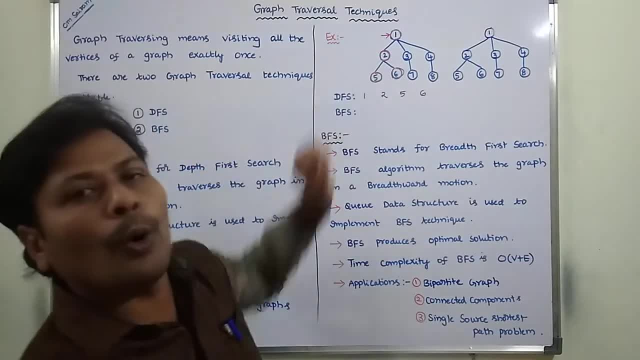 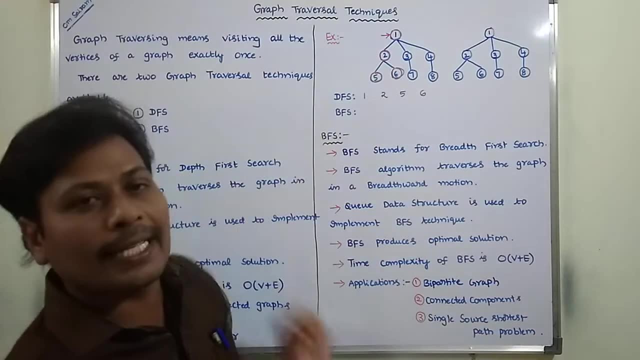 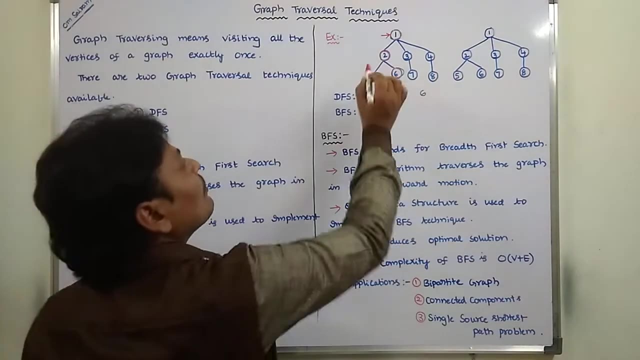 Next one. Then consider vertex 2.. There are no adjacent vertices for vertex 2.. That is, 1 is already visited, 5 is already visited, 6 is already visited. There are no unvisited adjacent vertices for vertex 2.. Again, we have to backtrack to vertex 1.. 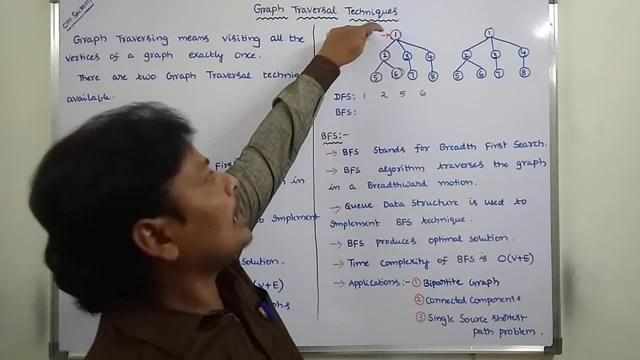 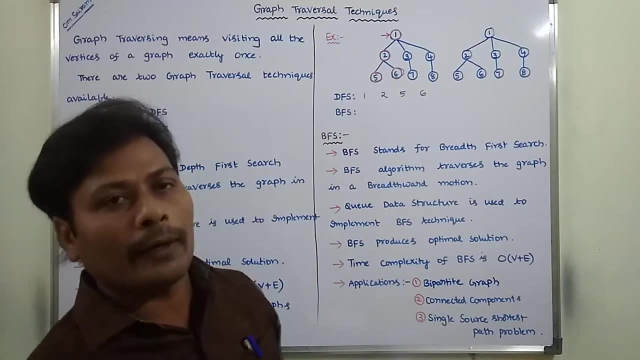 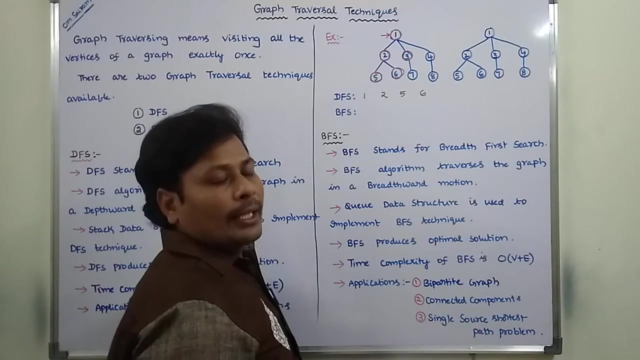 Now, what are the adjacent vertices for vertex 1?? 2, 3, 4.. Among them, vertex 2 is already visited, okay, Okay. the remaining two vertices, vertex 3 and vertex 4, are not visited, so that we have to take one vertex as visited among the vertex 3 and vertex 4.. 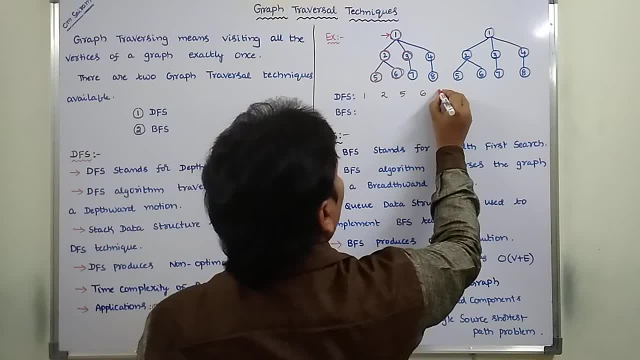 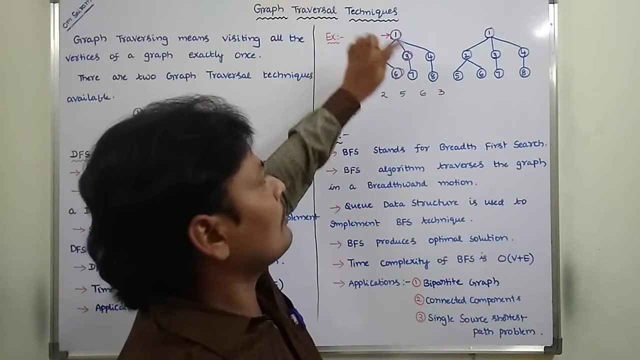 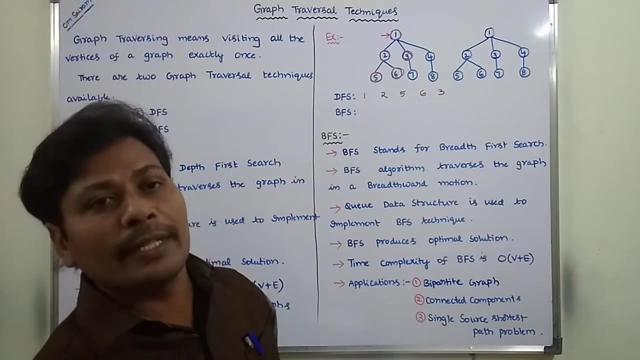 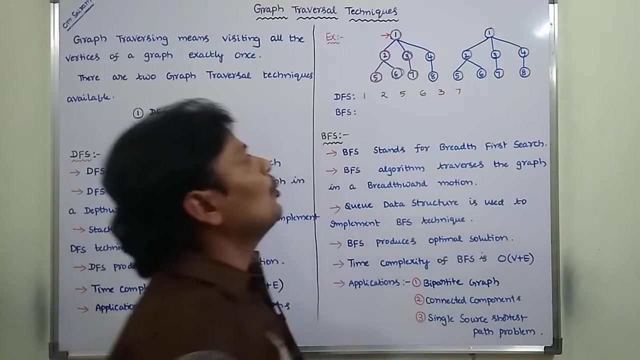 Now I am considering vertex 3, so that vertex is visited. Okay, now what are the adjacent vertices for vertex 3, vertex 1 and vertex 7. among them, vertex 1 is already visited, So vertex 7 is unvisited, so that we have to visit vertex 7 that is adjacent to vertex 3.. 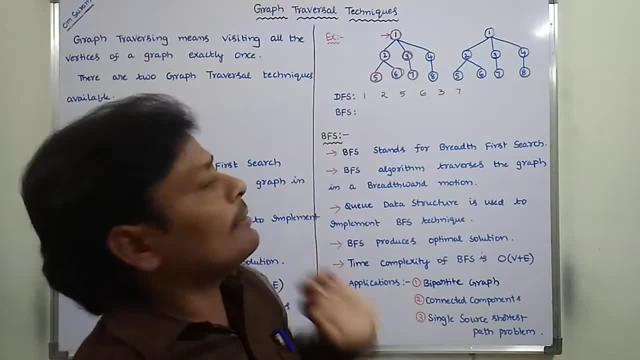 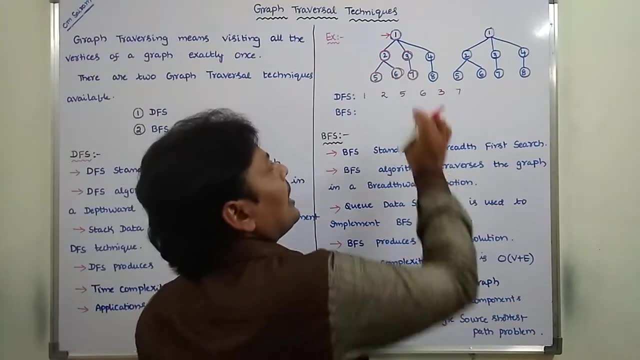 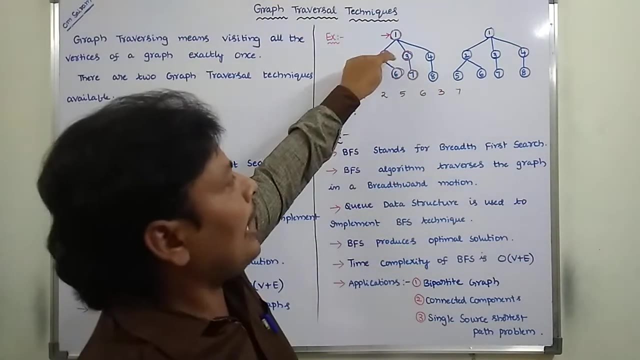 Okay, now what are the adjacent vertices for vertex 7,? only 3, but 3 is already visited. Okay, so there are no adjacent vertices for vertex 7.. Again, backtrack to vertex 3.. What are the adjacent vertices? Adjacent vertices for vertex 3, 1 and 7, but both are visited. 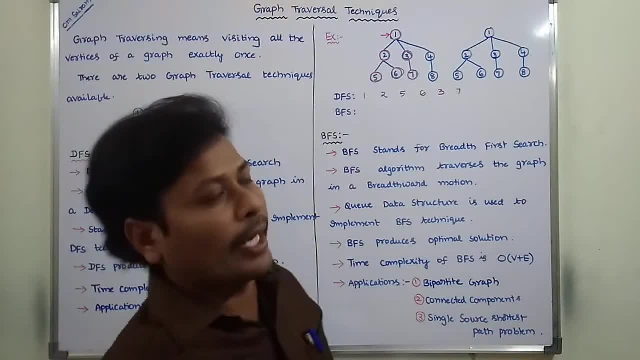 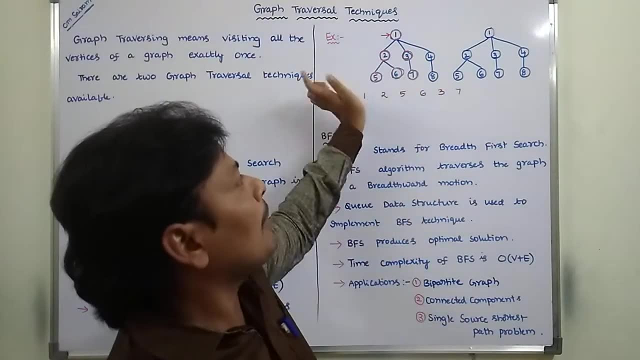 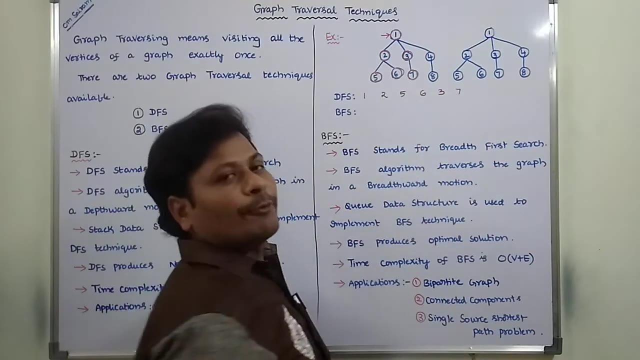 Okay, again we have to backtrack to vertex 1.. What are the adjacent vertices for vertex 1, vertex 2, vertex 3, vertex 4. among them, 2 and 3 vertices are already visited, So the remaining vertex 4 is not visited, so that I am taking vertex 4 as visited. 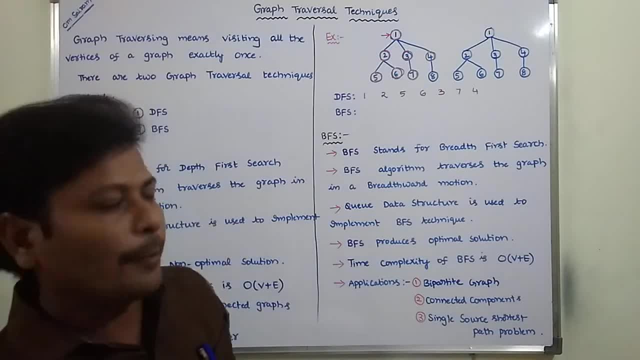 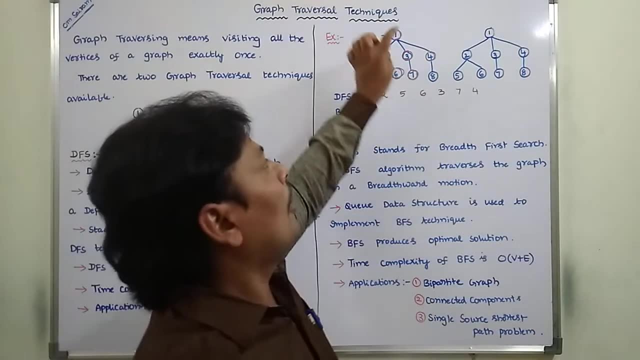 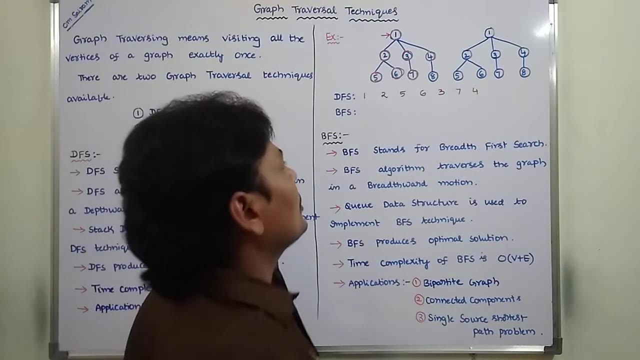 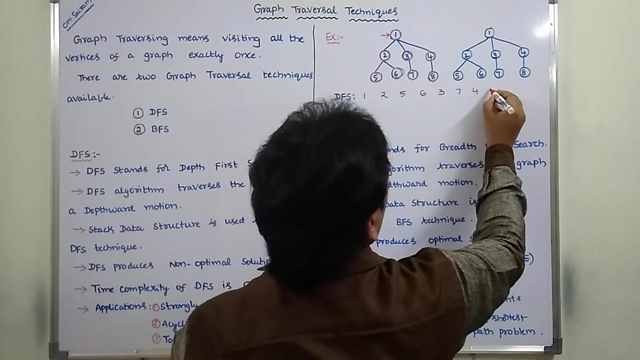 And it is adjacent to vertex 1.. Okay, now consider vertex 4.. What are the adjacent vertices for vertex 4, vertex 1 and vertex 8? among them, vertex 1 is already visited. Okay, so vertex 8 is not visited, so that vertex 8 is visited. that is adjacent to vertex 4.. 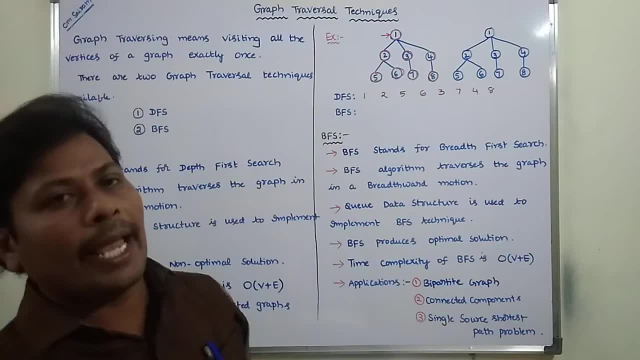 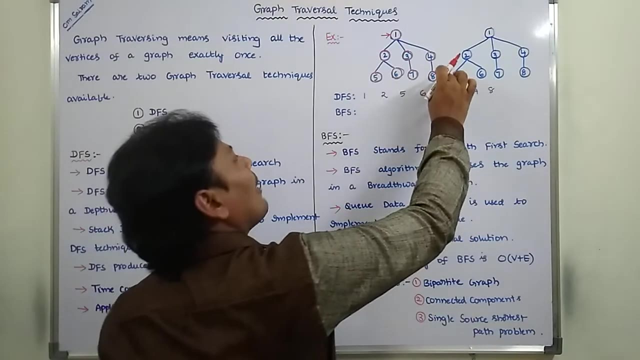 Okay, now consider vertex 8.. What are the adjacent vertices for vertex 8, vertex 4 only. but vertex 4 is already visited. There are no adjacent unvisited vertices for vertex 8.. Again, we have to backtrack to vertex 4.. 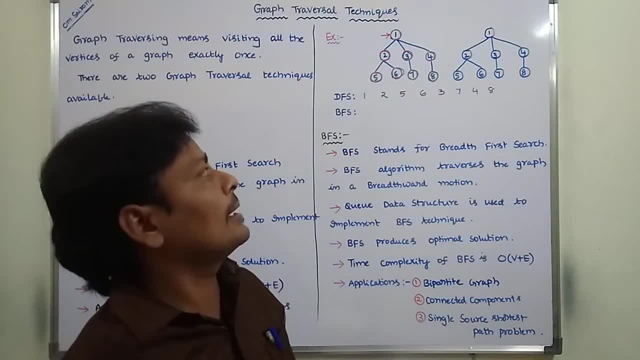 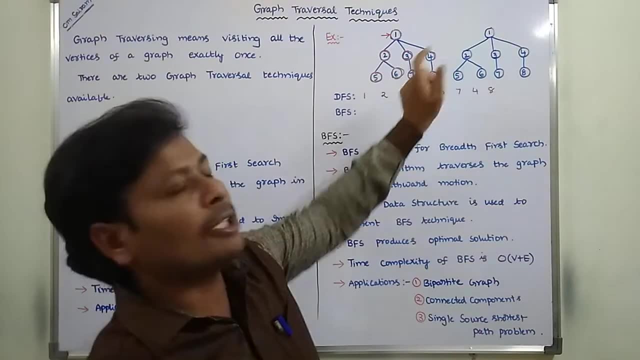 Next consider the vertex 4.. What are the adjacent vertices? are there 1 and 8? but both are visited. There are no adjacent unvisited vertices for vertex 4.. Now again, we have to backtrack to vertex 4.. Again, backtrack to vertex 1.. 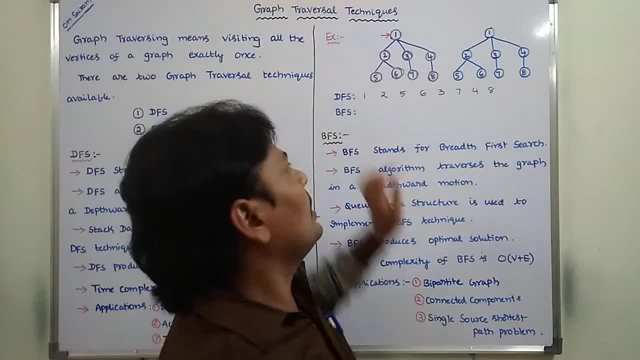 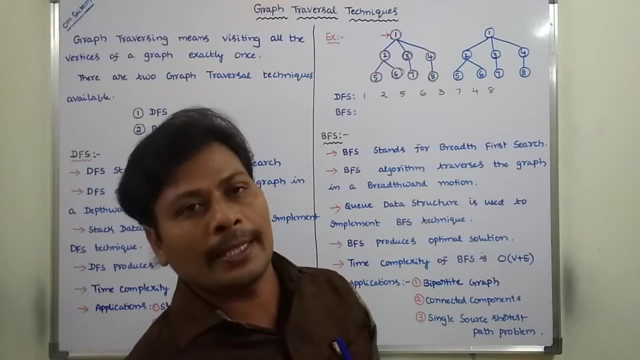 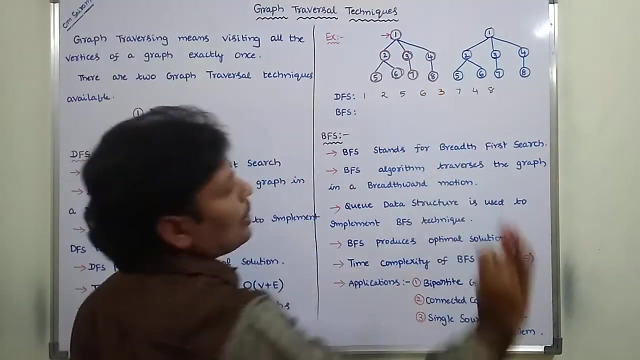 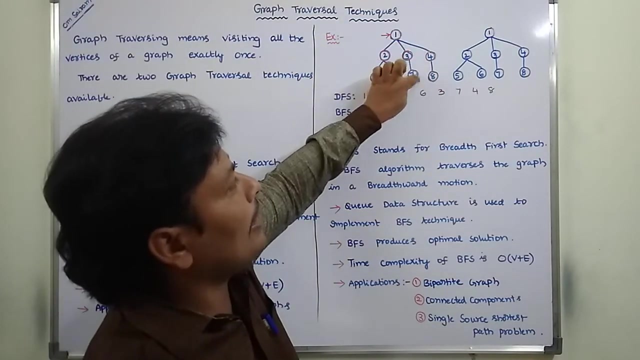 So what are the adjacent vertices for vertex 1, 2, 3, 4.. Already 3 vertices are visited. There are no unvisited vertices for vertex 1 that is adjacent. So again we have to stop that procedure. So 1, 2,, 5, 6, 3, 7,, 4, 6.. 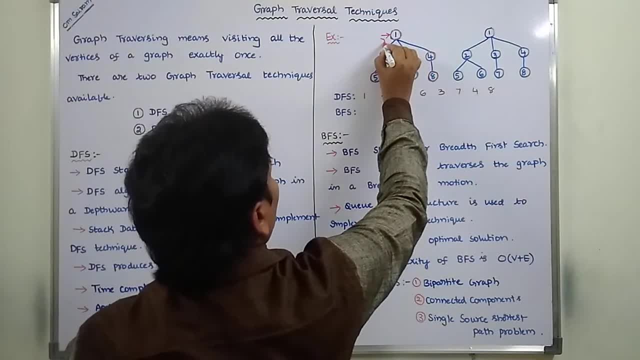 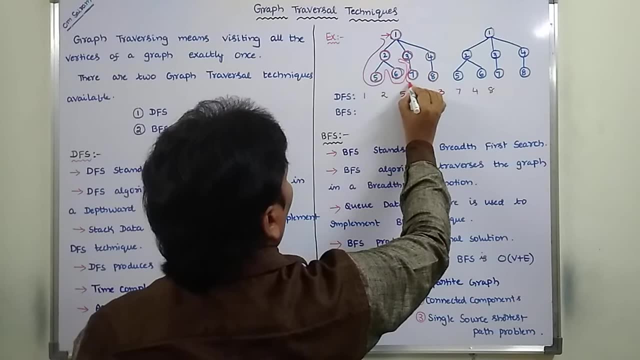 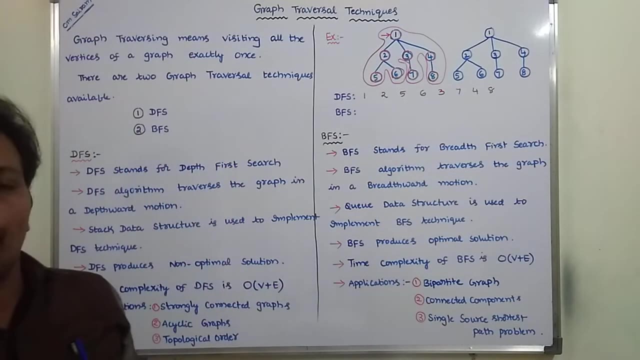 So this is the vertex 4.. So this is the depth word motion. This is called as the depth word motion. Okay, next one. Stack data structure is used to implement the DFS technique. Okay, next one: DFS. DFS produces non-optimal solution, whereas DFS produces optimal solution because DFS produces a spanning tree. it produces the optimal solution when we are considering the single source shortest path problem, but DFS produces a DFS spanning tree. 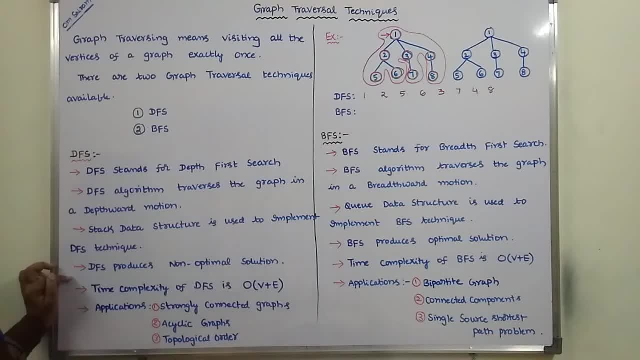 So that is not a optimal solution. So that is not a optimal solution. So because of that reason DFS produces non-optimal solution Next time. complexity of DFS is big O of V plus E. So V is nothing but set of vertices, E is nothing but set of edges. 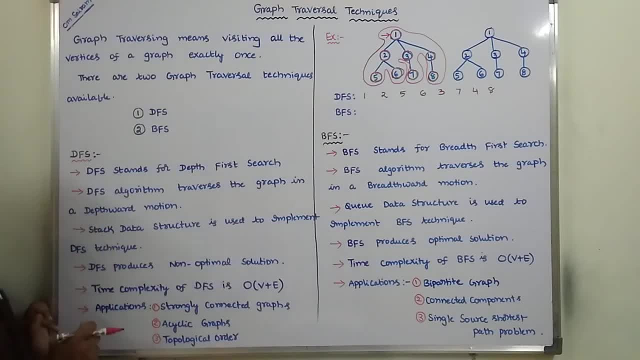 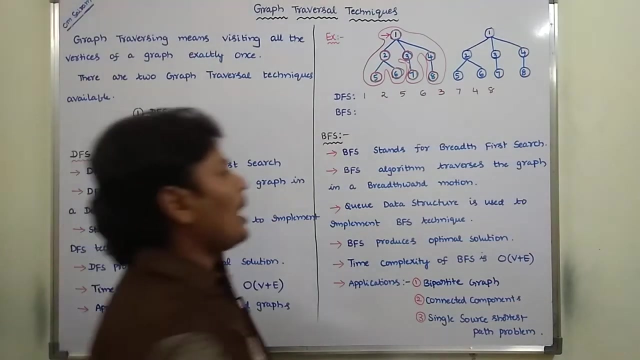 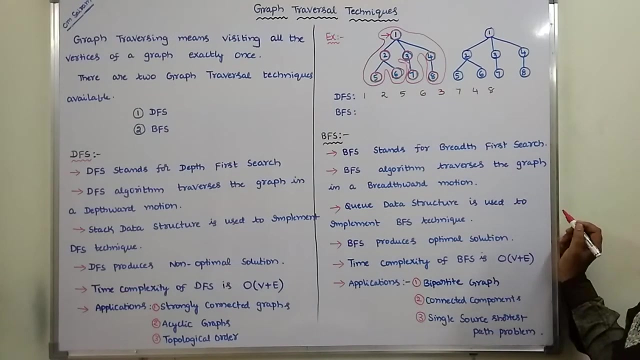 Next one, Applications of DFS, is strongly connected components, acyclic graphs and topological order. So in these three applications we have to use depth, first, search technique, Next. Now go for BFS. BFS stands for breadth, first, search technique. Next, BFS algorithm traverses the graph in a breadth word motion. 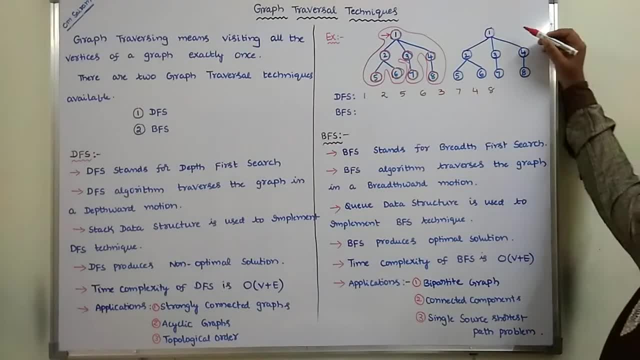 What is breadth word motion In the BFS. In the BFS, Visiting all the words in the graph In the BFS, Visiting all the words in the graph. Visiting all the words in the graph. Visiting all the words in the graph. 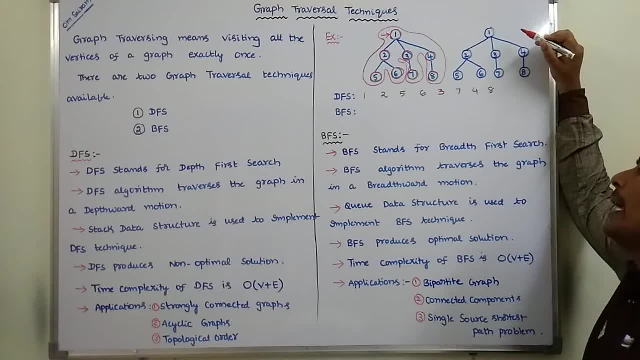 Visiting all the vertices in a level by level order. Okay, Here breadth word motion means visiting all the vertices in a level by level order. So this is level 1 and this is level 2 and this is level 3.. First, we have to visit all the vertices in level 1.. 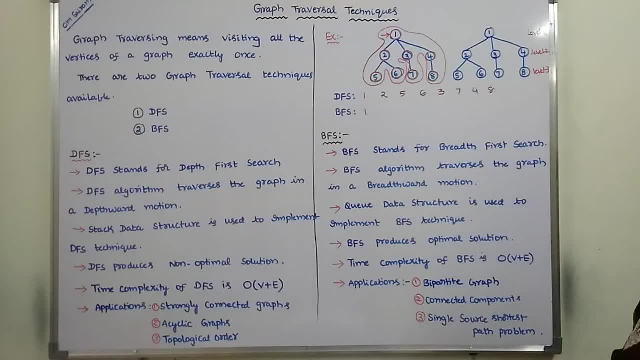 In the level 1, only one vertex is there that is visiting Next one In level 2.. There are three vertices are there? Three vertices are visiting, So 2., 3., 4.. Okay, Next in level 3.. 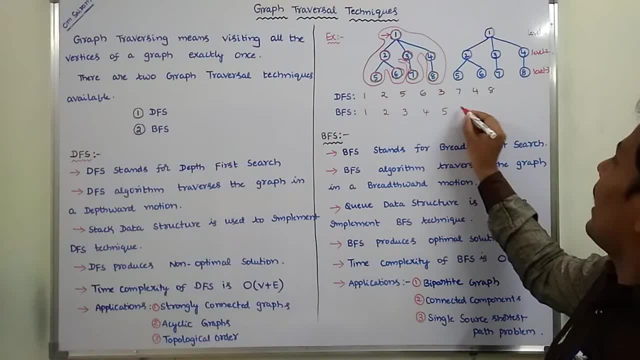 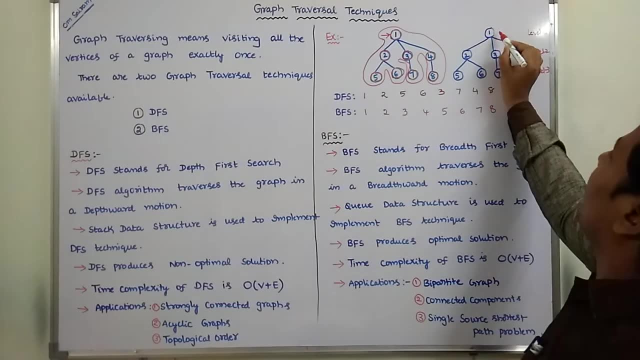 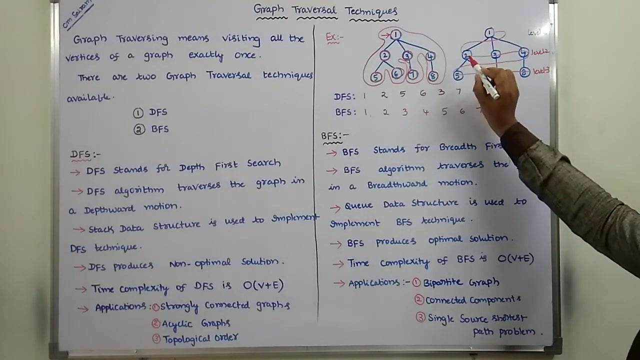 There are three vertices are there that are visited: 5., 6., 7. 8.. Okay, So this is called as level-by-level order. This is called as level by level order, So this is called. 1 contains vertex 1 that is already visited. level 2 contains 3 vertices: 2, 3, 4 that is already visited. 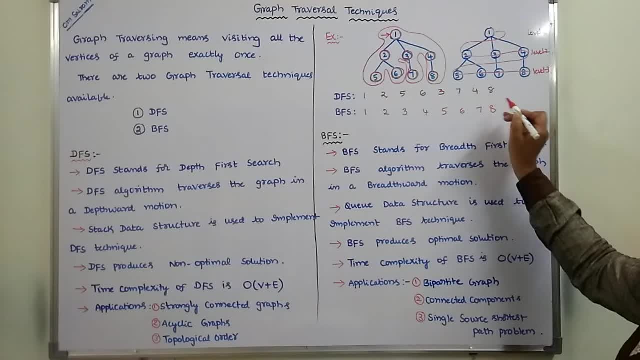 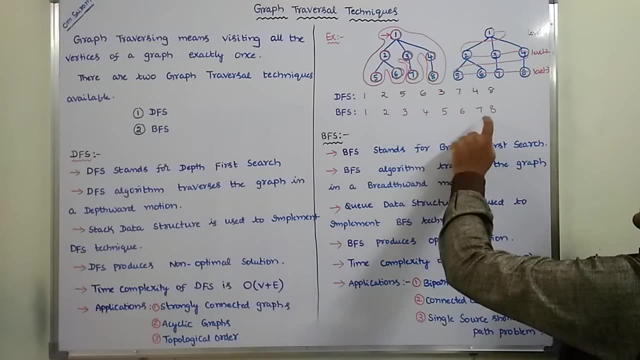 level 3 contains 3 vertices: 5, 6, 7, 8. that is already visited, so that bfs order is 1, 2, 3, 4, 5, 6, 7, 8. okay, next one q data structure is used to implement bread first. such picnic, okay. 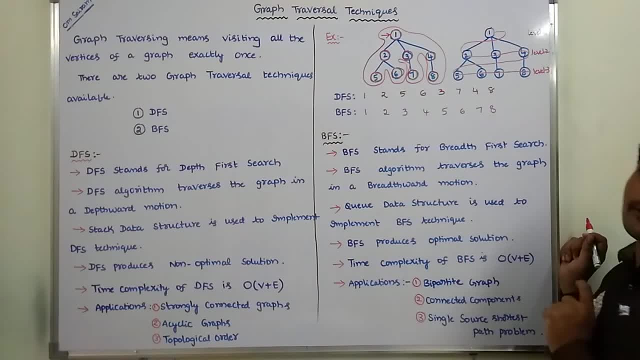 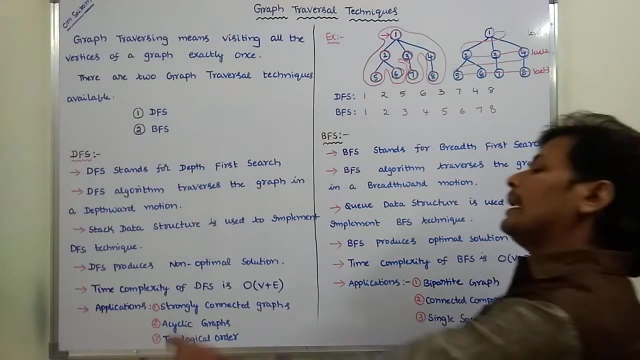 next one, bfs, produces a optimal solution. so in the case of bfs, the output of bfs is bfs spanning tree. that spanning tree produces the shortest path between shortest path between source vertex to remaining all the vertices of a given graph. okay, so then BFS produces a optimal solution, whereas DFS does not produce any optimal. 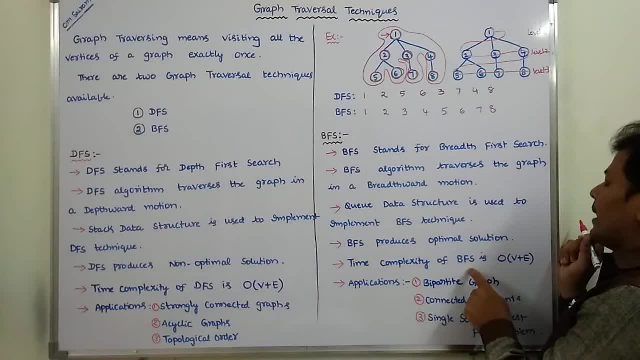 solution. next, the time. complexity of BFS is big O, where B is the set of vertices and D is the set of edges. next, wait, this application of BFS is bipartiழ graph, okay. second one is connected components. third one is single source. shortest path problem, okay, whatever. thus spanning tree we are. 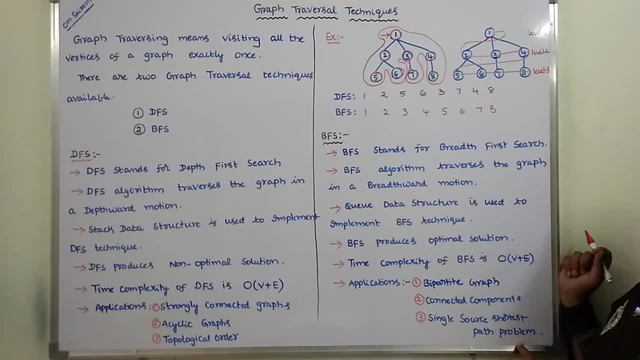 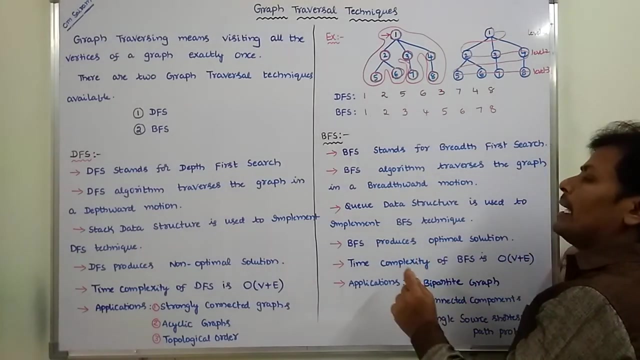 br embedded that spanning tree can be treated as the shortest path between source vertex to remaining all the vertices. so it is determines only converter. we have a transportationrios in. we can simply put Geoffrey as a path, only not the cost. okay, so because of the treason, BFS produces a optimal.